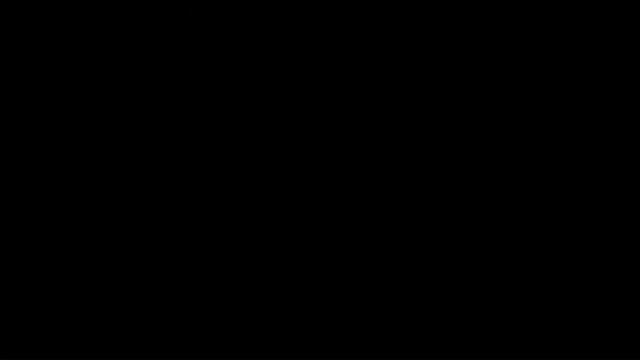 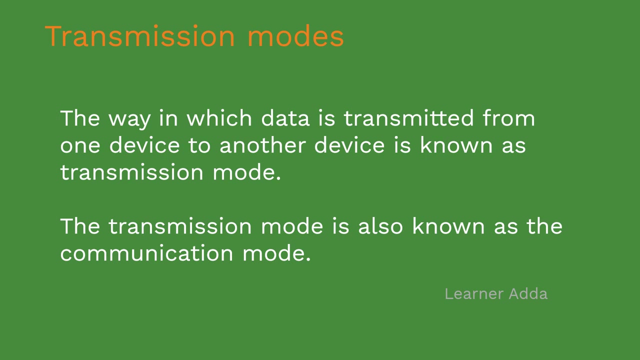 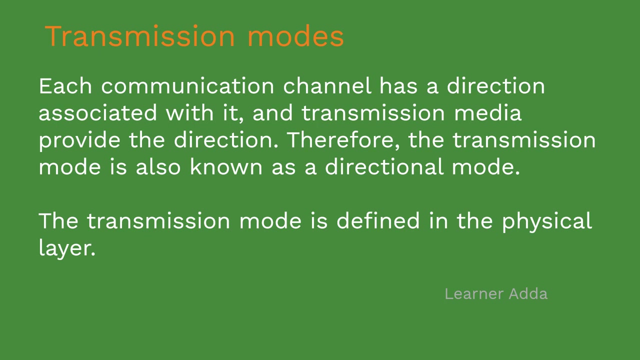 Transmission modes. The way in which data is transmitted from one device to another device is known as transmission mode. The transmission mode is also known as the communication mode. Each communication channel has a direction associated with it and transmission media provide the direction. Therefore, the transmission mode is also known as a directional mode. 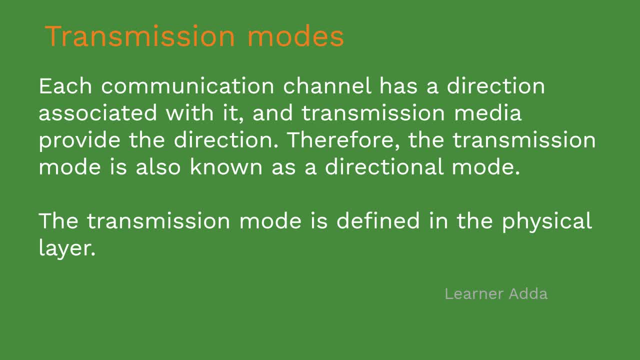 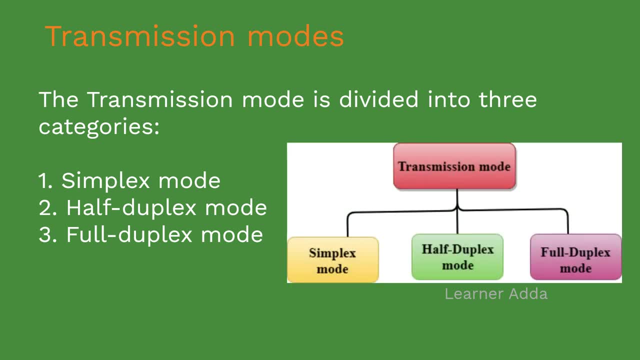 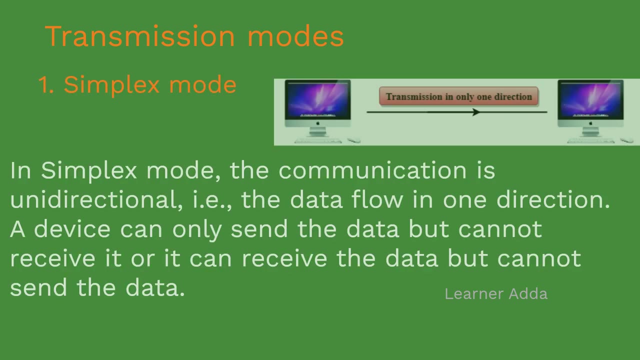 The transmission mode is defined in the physical layer. The transmission mode is divided into three categories: Synthlex mode, Half duplex mode, Full duplex mode. Synthlex mode. In synthlex mode the communication is unidirectional, ie the data flow in one direction. A device can only send the data, but 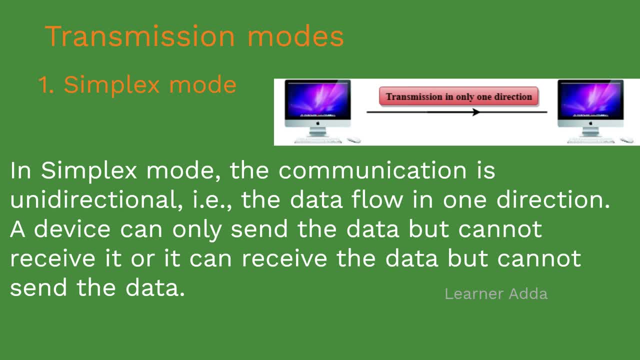 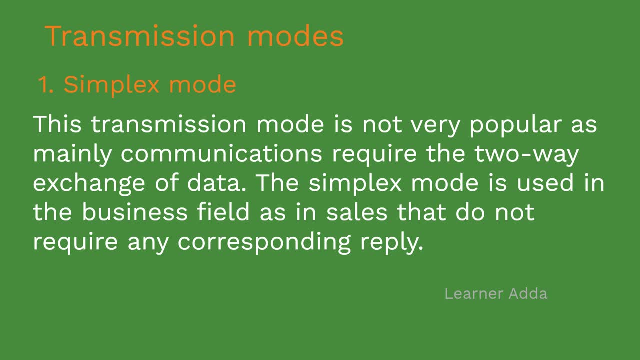 cannot receive it, or it can receive the data but cannot send the data. This transmission mode is not very popular as mainly communications require the two-way exchange of data. The synthlex mode is used in the business field, as in sales that do not require any kind of communication. The transmission mode is used in the business field, as in sales that do not require any kind of communication. 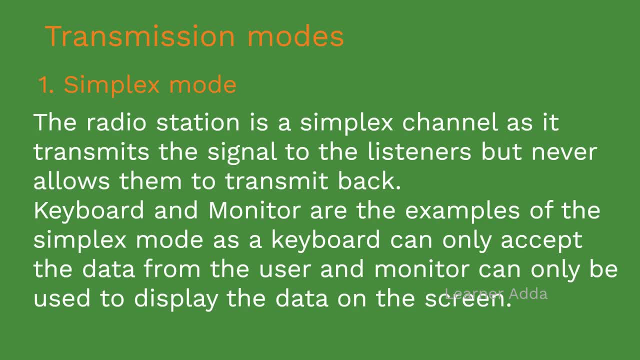 Any corresponding reply. The radio station is a synthlex channel, as it transmits the signal to the listeners but never allows them to transmit back. Keyboard and monitor are the examples of the synthlex mode, as a keyboard can only accept the data from the user and monitor can only be used. 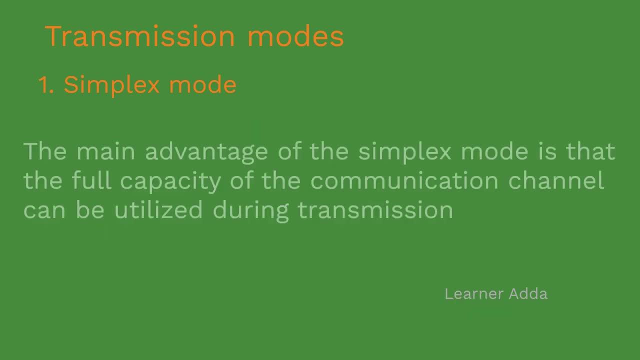 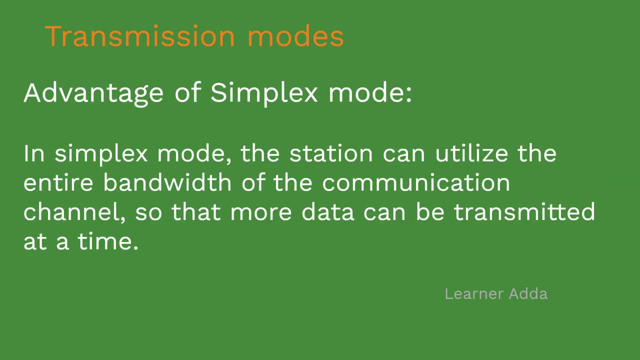 to display the data on the screen. The main advantage of the synthlex mode is that the full capacity of the communication channel can be utilized during transmission. Advantage of synthlex mode: In synthlex mode, the station can utilize the entire bandwidth of the. 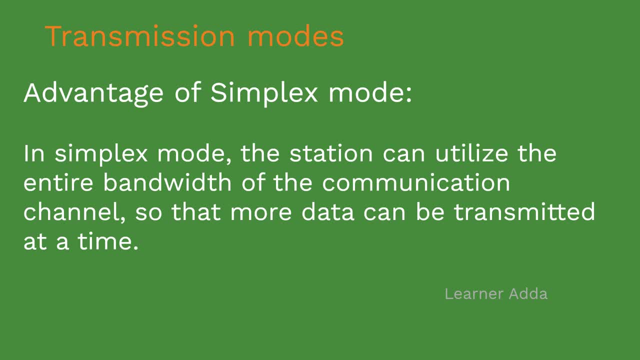 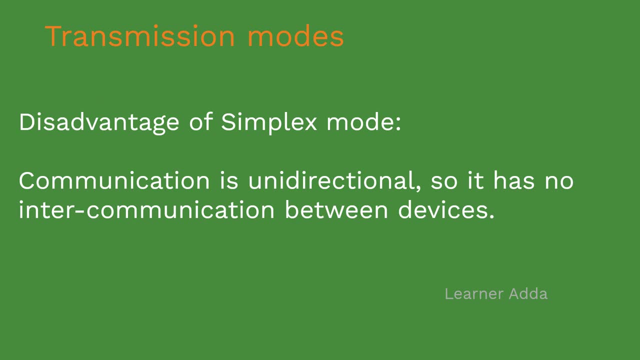 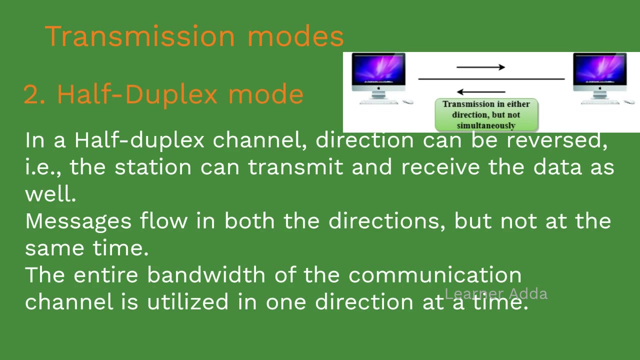 communication channel so that more data can be transmitted at a time. Disadvantage of synthlex mode: Communication is unidirectional, so it has no intercommunication between devices. Huff duplex mode. In a huff duplex channel direction can be reversed, ie the station. 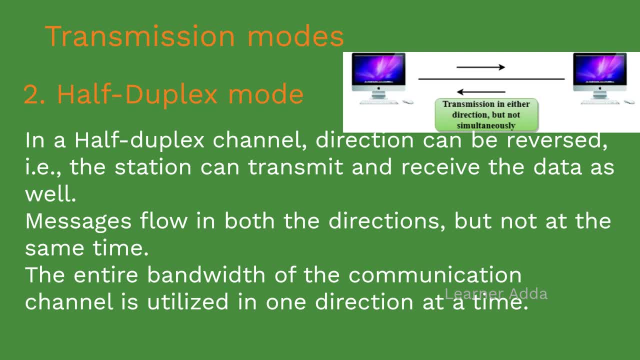 can transmit and receive the data as well. Messages flow in both the directions, but not at the same time. The entire bandwidth of the communication channel is utilized in one direction at a time. In huff duplex mode, it is possible to perform follow-up communications with. the signal and not the signal with which the signal is sent or the signal is sent according to the direction of the transmission. The Cynthia's example offers an intermediate experience Of tinha 2.. I also have an hills nickname. The cypress grew, but the sound was too loud to hear. I have been in the agricultural field for far a generation. 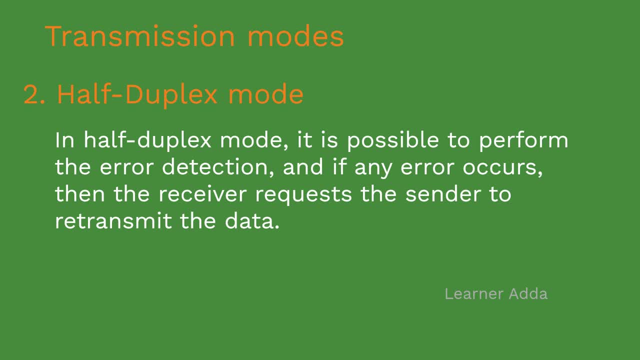 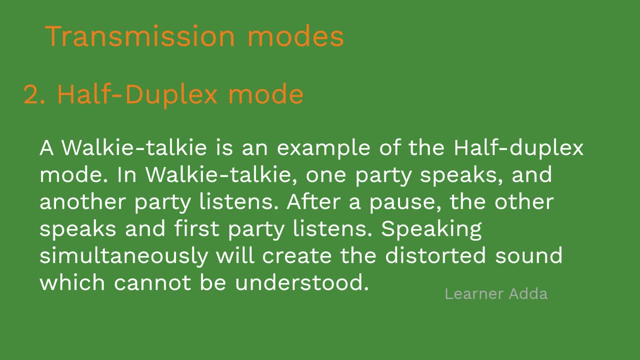 the error detection and if any error occurs, then the receiver requests the sender to retransmit the data. A walkie-talkie is an example of the half-duplex mode. In walkie-talkie one party speaks and another party listens. After a pause, the other speaks and first party listens. 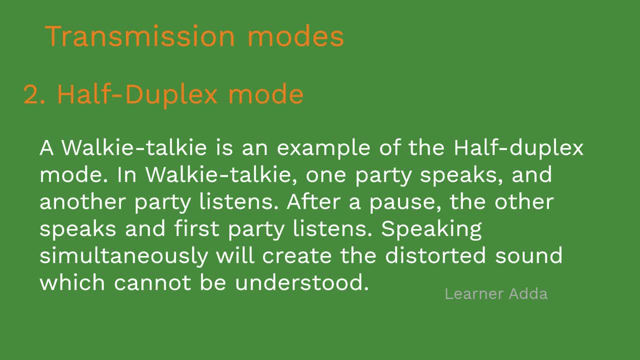 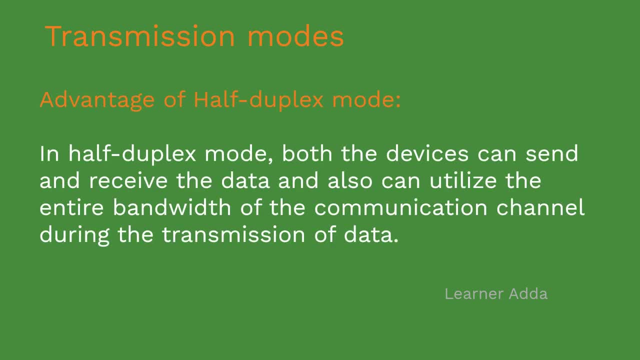 Speaking simultaneously will create the distorted sound which cannot be understood. Advantage of half-duplex mode: In half-duplex mode, both the devices can send and receive the data and also can utilize the entire bandwidth of the communication channel during the transmission of data. Disadvantage of half-duplex mode: In half-duplex mode: 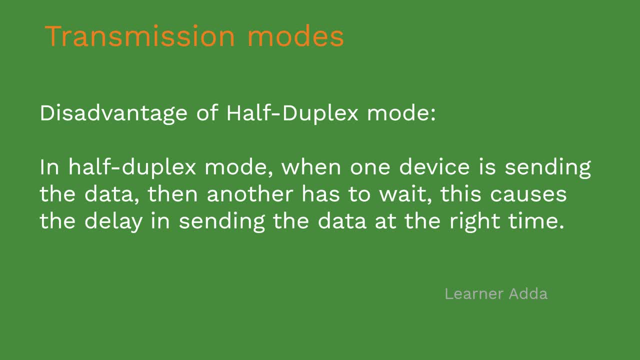 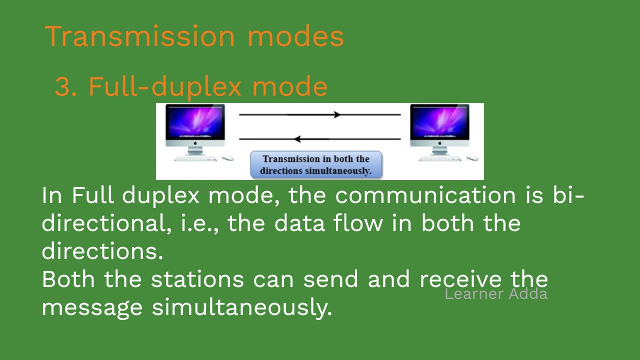 when one device is sending the data, then another has to wait. This causes the delay in sending the data at the right time. Full-duplex mode. In full-duplex mode, the communication is bi-directional, ie the data flow in both the directions. 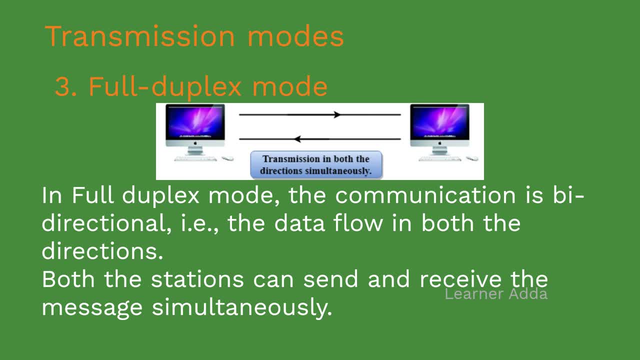 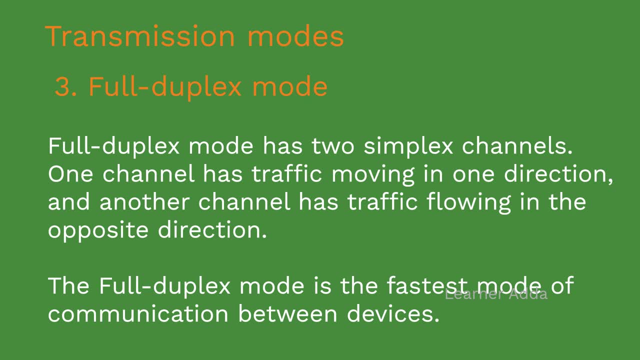 Both the stations can send and receive the message simultaneously. Full-duplex mode channels. One channel has traffic moving in one direction and another channel has traffic flowing in the opposite direction. The full duplex mode is the fastest mode of communication between devices. 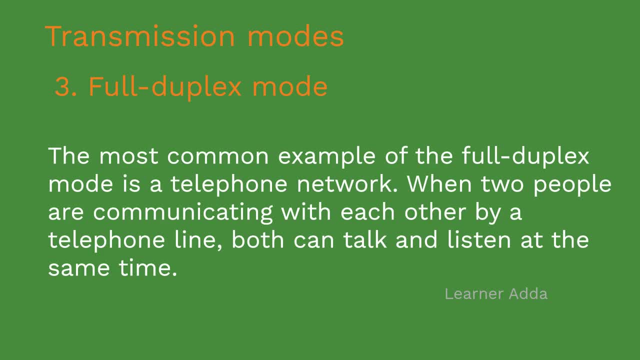 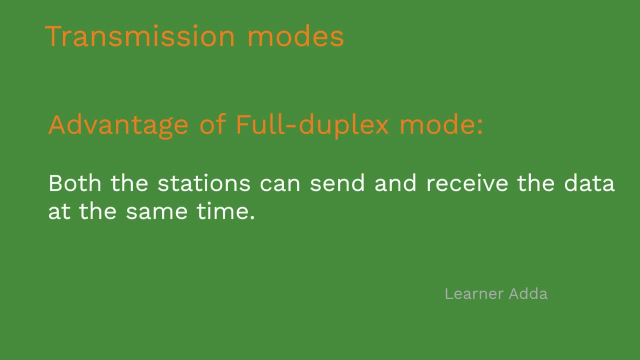 The most common example of the full duplex mode is a telephone network. When two people are communicating with each other by a telephone line, both can talk and listen at the same time. Advantage of full duplex mode: Both the stations can send and receive the data at the same time.